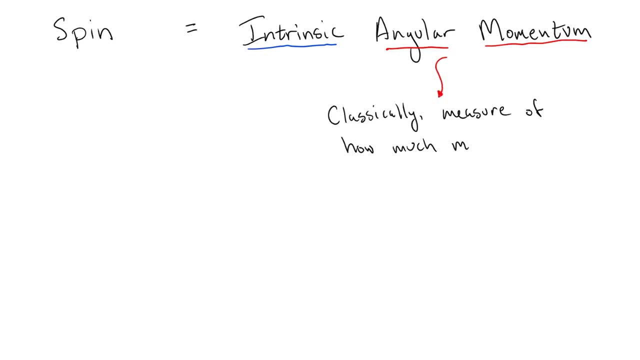 we can think of classically as a measure of how much motion an object has around a given axis. This is usually the case for a particle spinning around an axis like a top. This is usually the split between two contributions: The contribution where the axis goes through the center of mass of. 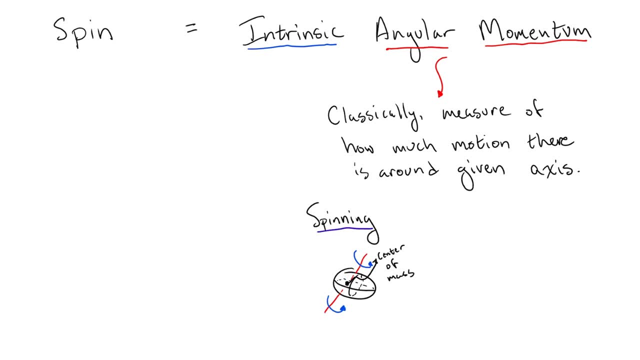 the object, which we can call the angular momentum from spinning, and the contribution where the axis is located outside the center of mass, called the orbital angular momentum. So, for example, the earth has some angular momentum associated to the fact that it's spinning around an axis. 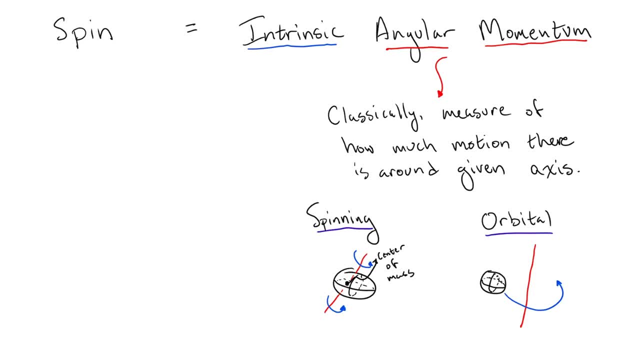 as well as the angular momentum it has from orbiting the sun. Here we see why it doesn't make sense to talk about a point particle spinning. If the particle is truly a point, then it's always located at its own center of mass. 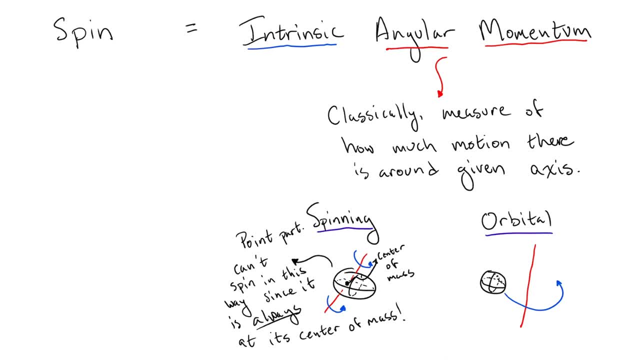 and so it can never have any motion around its center of mass. Therefore a point particle can't have classical angular momentum from spinning, though it can still have orbital angular momentum. The other important piece of quantum spin is the intrinsic part. This is 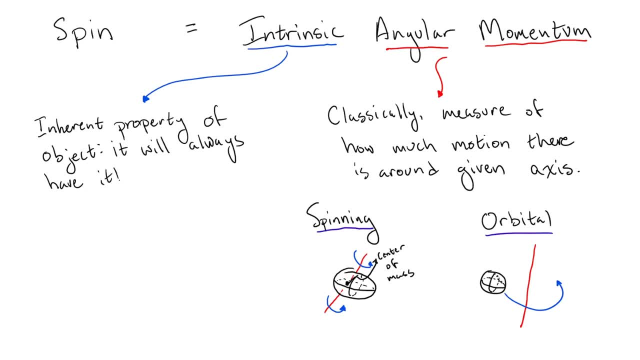 simply a function of the angular momentum. This simply means that anything with quantum spin just has angular momentum, regardless of whether or not it is classically spinning or orbiting. This may seem a little strange at first. After all, how can something which is sitting completely 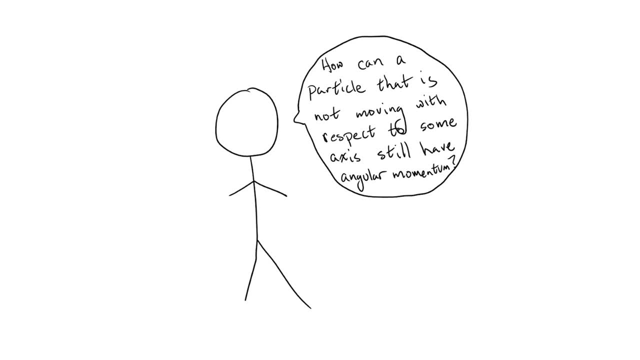 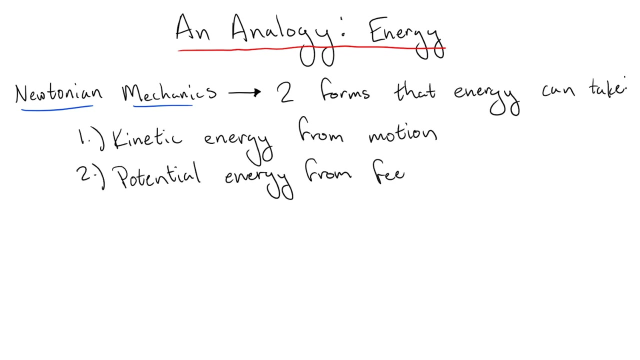 still in free space have non-zero angular momentum. But it turns out that there's a great analogy that many people will be more comfortable with. In Newtonian mechanics, a particle can only have energy if it's moving. When we upgrade our picture to use special relativity, 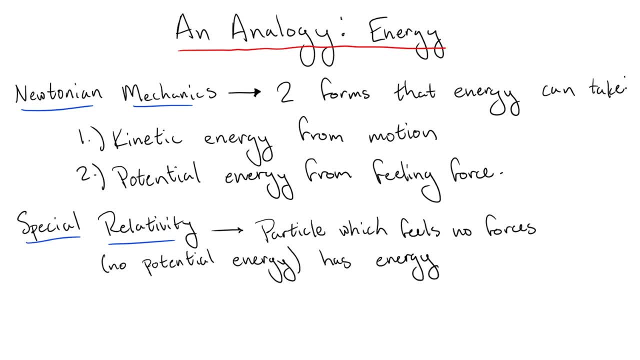 we find the famous equation for the energy of a free particle- meaning it doesn't experience any forces- Which, in the case that the particle is not moving, simply becomes E equals mc squared. But this is saying that a particle which is feeling no forces and is not moving, 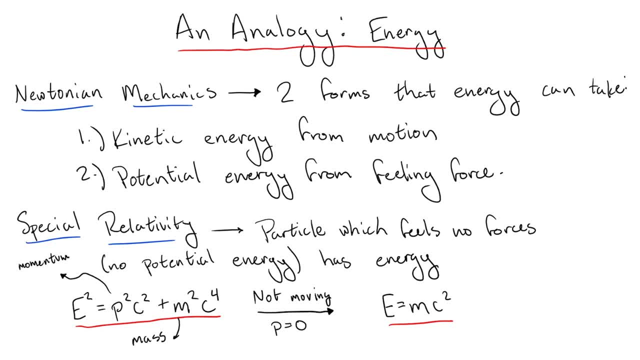 has energy to it, completely counter to what we find in the Newtonian case. But in other words, massive particles have intrinsic energy. So if we want to create a massive particle, it will cost us energy to do so. Spin is exactly analogous. When we use quantum mechanics we can have point particles. 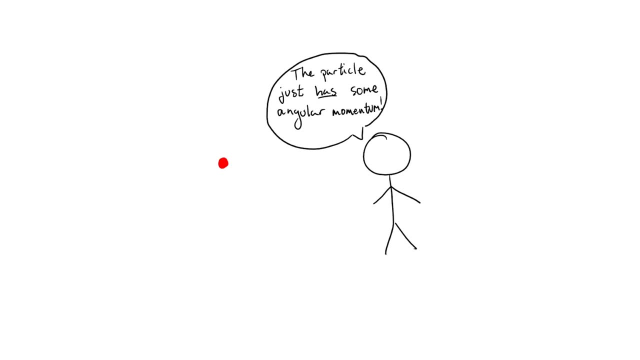 which are completely stationary, that still have some angular momentum, And if we want to create such particles, it will cost us that amount of angular momentum to do so. This amount of angular momentum is the particle's quantum spin. Now it's very important not to get this classical spinning angular momentum mixed up with quantum. 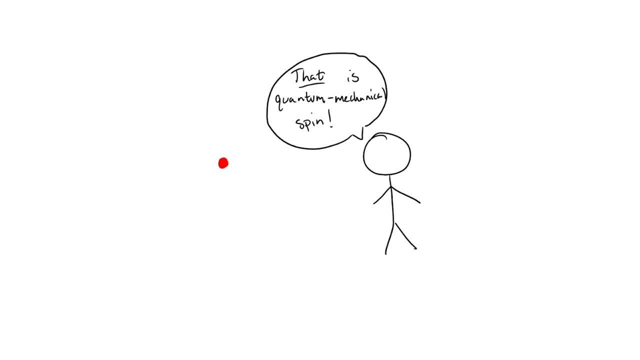 mechanical spin, since they are incredibly different. To hopefully avoid any confusion from this point forward, when we refer to just spin we'll be talking about intrinsic angular momentum from quantum mechanics, and if we want to talk about the classical version, we will. 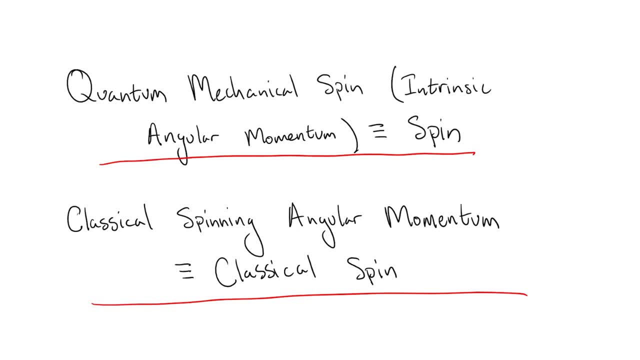 explicitly refer to it as spin, And then we will talk about quantum mechanics, which is a quantum to it as classical spin. Okay, so now that we have an idea of what spin is, we can ask what values this spin can take. To figure this out, we need two facts. 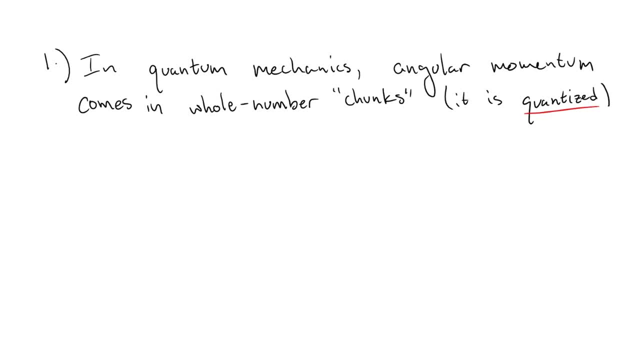 The first is that any form of angular momentum, either spin or orbital, in quantum mechanics is quantized, meaning that it comes in whole number units. The second fact is that the quantum mechanical properties of angular momentum are deeply tied to those of rotations. 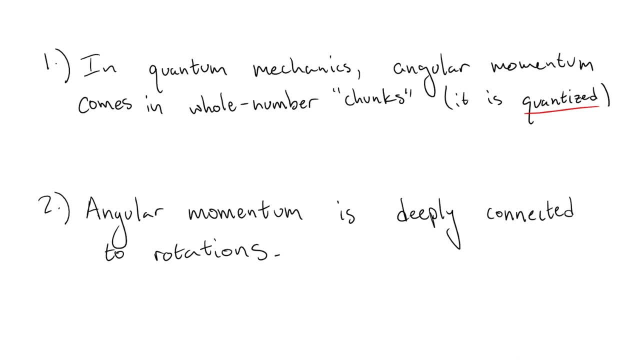 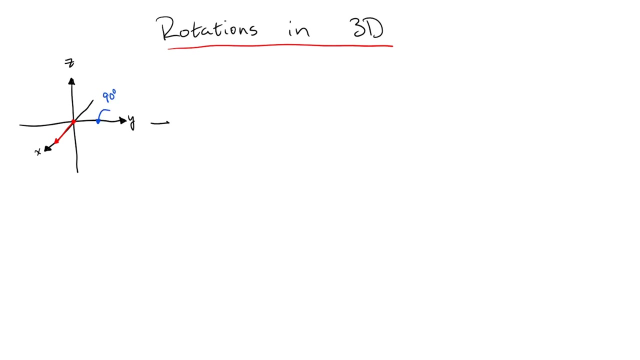 This latter point is incredibly important due to the fact that rotations in three dimensions have the special property that their order matters. Consider an arrow in three-dimensional space, initially pointing along the positive x-axis, Then rotate the arrow by 90 degrees around the y-axis, then rotate by 90 degrees around. 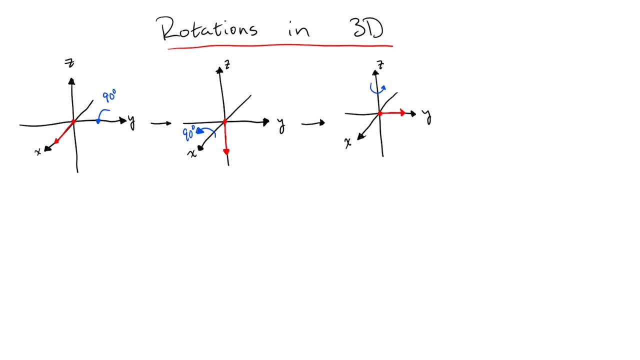 the x-axis and finally rotate by 90 degrees around the y-axis. After all of this, the arrow is now pointing in the negative x-direction. Now we will again start with the arrow pointing in the positive x-direction, but instead first rotate by 90 degrees around the z-axis, then 90 degrees about the x-axis and finally 90. 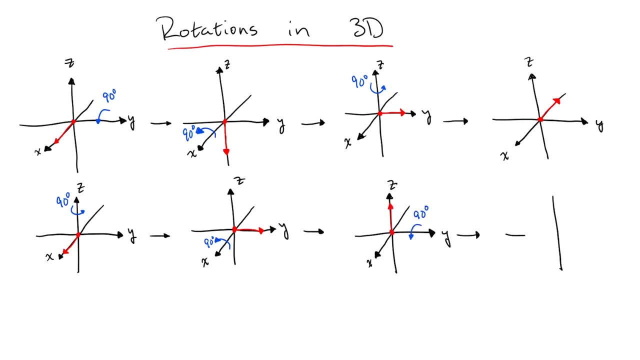 degrees about the y-axis. Here we should find that the arrow is pointing in the positive x-direction. In each of the two cases we use the positive x-direction. We used the exact same rotations but in a different order, and found that the final 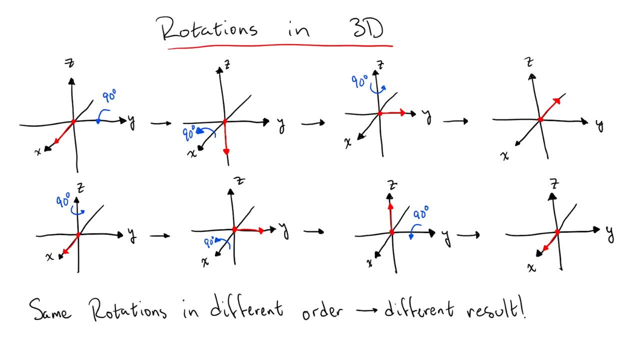 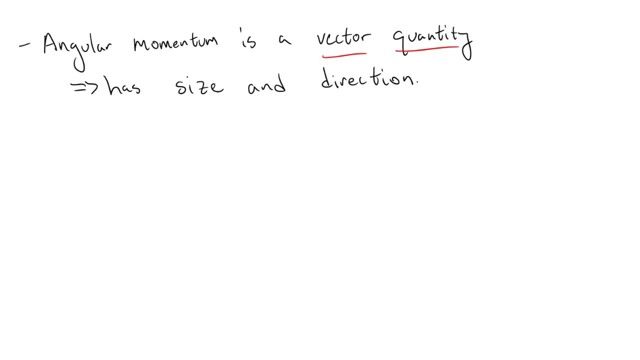 states are completely different. So what does this mean for angular momentum? Well, angular momentum is a vector quantity, which means that it has both size and direction. Since the order of rotations about each of our independent directions mattered, this property carries over to measurements of angular momentum in quantum mechanics. 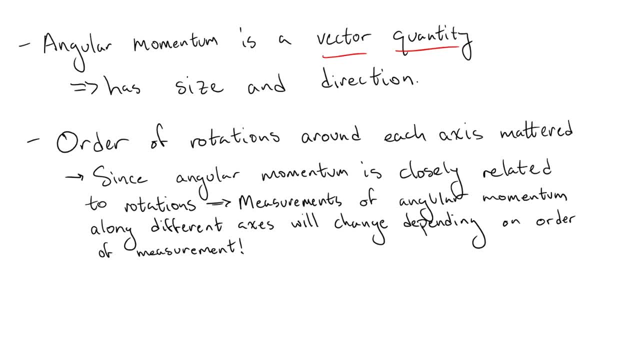 If we measure the angular momentum of a state in x-direction, we can measure the angular the x direction and then in the z direction. we will get a different answer than if we measure the angular momentum in the z direction and then in the x direction. 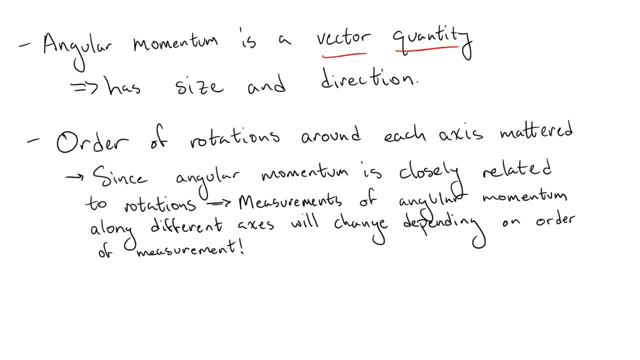 In more technical terms, we would say that the components of the angular momentum operator do not commute. The result of this non-commutation is that we are only allowed to know the components of angular momentum in a single direction and are forced into complete ignorance about. 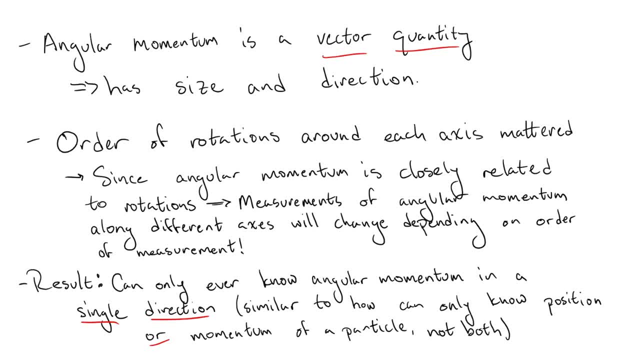 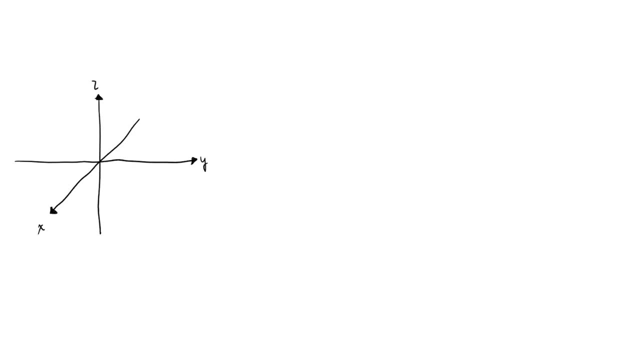 the other components. Note that this is almost exactly the same story as measurements of position and momentum. We can know one or the other, but never both. So this means that we can know the total magnitude as well as a single component of the direction. 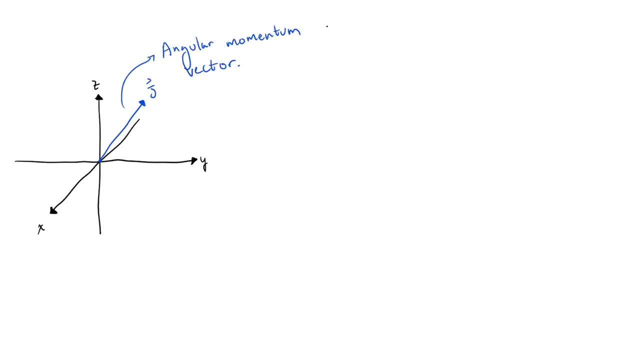 of the angular momentum of the state. We could choose any direction we want, but conventionally the z direction is often chosen. We will write this z component of angular momentum as a product of a constant with units of angular momentum called h-bar times, some number. 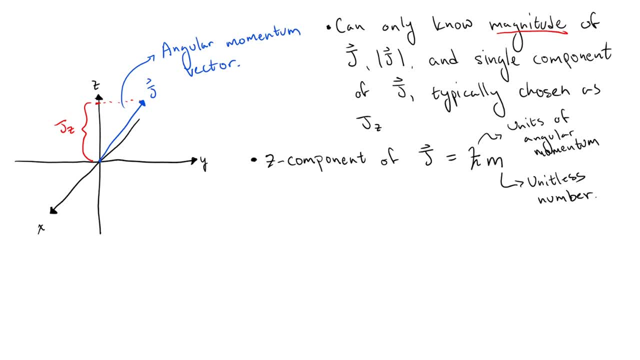 which we will call m. Now, since the z component of the angular momentum will have a maximum value, there will be a max value that m can take, which we will call l. A subtlety here is that h-bar times l is not exactly equal to the total magnitude of the. 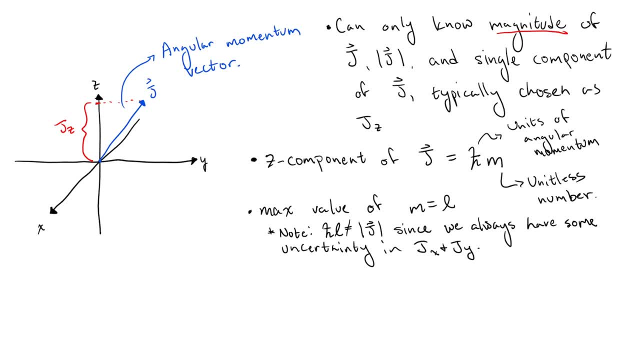 angular momentum. due to the fact that there is always some uncertainty in the angular momentum in the x direction, This means that we have to always allocate some of the total magnitude in these directions. So h-bar l will always be a little bit less than the total magnitude of the angular momentum. 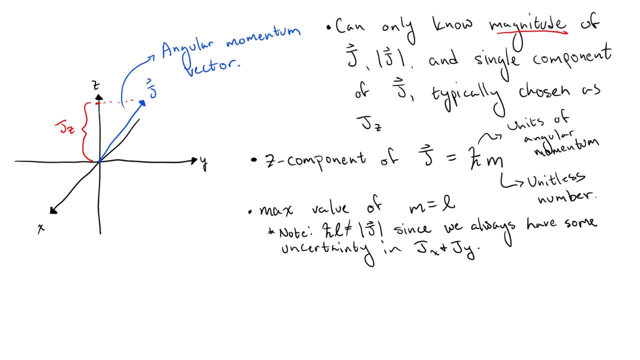 of the state. This maximum value of m will be when the most angular momentum we can have in the z direction is pointed along the positive z axis. However, this angular momentum can, of course, also point in the negative direction, As we already established, there's nothing really special about the axis that we choose. 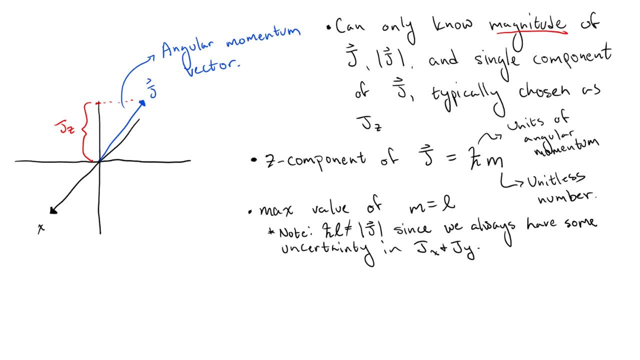 so it shouldn't matter how we pick the positive or negative axes. So if we have a maximum value for m of l in the positive z direction, we should also have a minimum value of minus l in the negative z direction. All in all, this means that m is bounded to be between minus l and l. 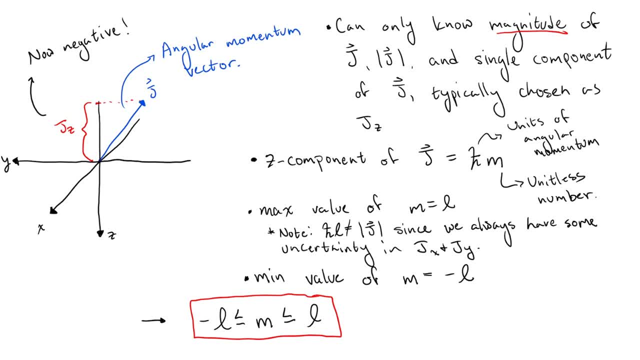 Here's where the fact that angular momentum is important. Let's take a look at an example of angular momentum in the negative z direction. Here's where the fact that angular momentum is bounded to be between minus l and l is quantized, comes into play. 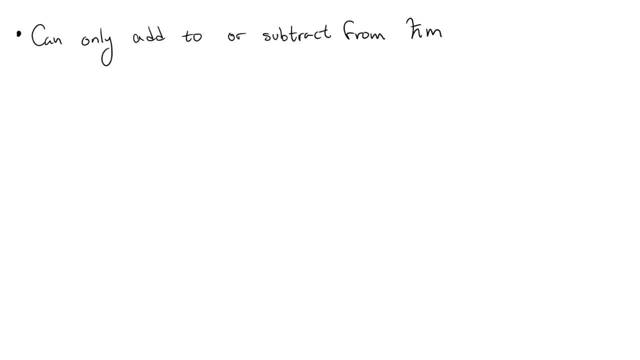 This quantization means that we can only add or subtract from h-bar times m chunks of angular momentum, each of which has size. h-bar Said in another way, we can only change m by integer values. So let's start with m equals minus l and add n units of h-bar until we get to m equals. 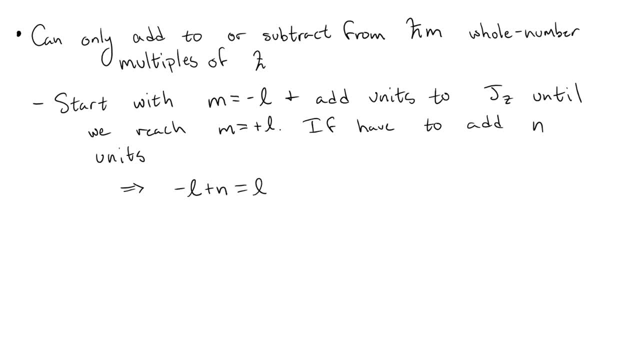 l. Then we find this equation Which we can solve. for l We'll define that l is equal to n over 2.. So we see only two options. The first is when n is even, in which case l is an integer. 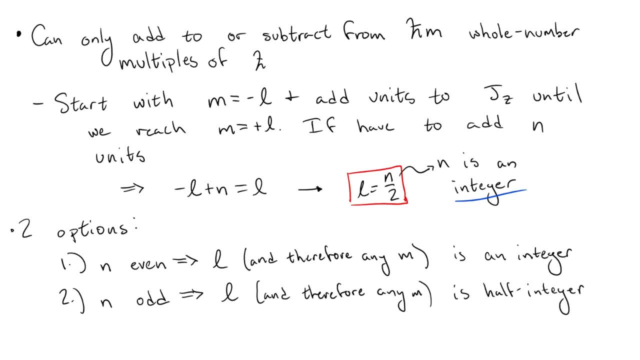 And the second is when n is odd and l is a half integer. Note that if l is an integer, any choice of m will also be an integer and the same for half integer values. This is the statement that the spin of a particle can only take integer or half integer values. 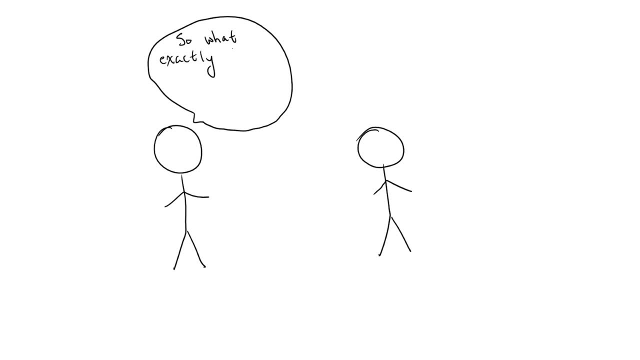 OK, So we have the possible spin states for a particle, but what exactly determines what spin state goes with which particle? To answer this question, we need to dip our toes into the realms of quantum field theory. Generic quantum-field theories are built to obey to the symmetries of special relativity. 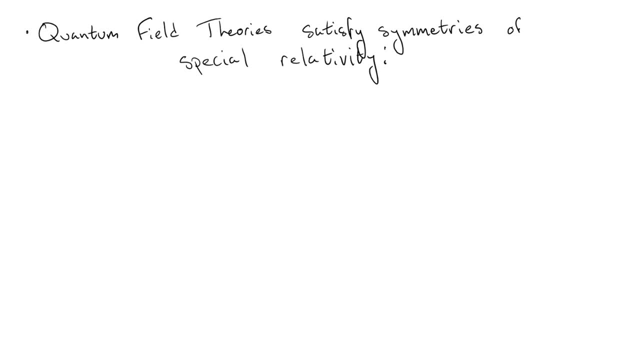 In particular, quantum fields transform under the combinations of Lorentz–transformations, translations and rotations, collectively called the Poincaré equations, collectively called the Poincaré group, where different quantum fields will transform differently under the Poincaré group. What we typically associate with a particle is an. 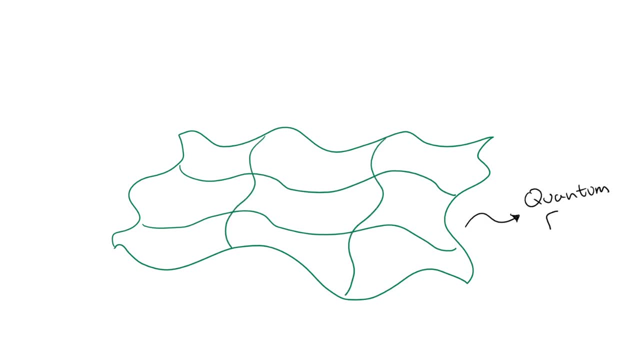 excitation of such a quantum field, so we can build a single particle state by exciting the vacuum state of the field. This is done mathematically with an object known as a field operator, which is defined at the point where we are creating the particle. 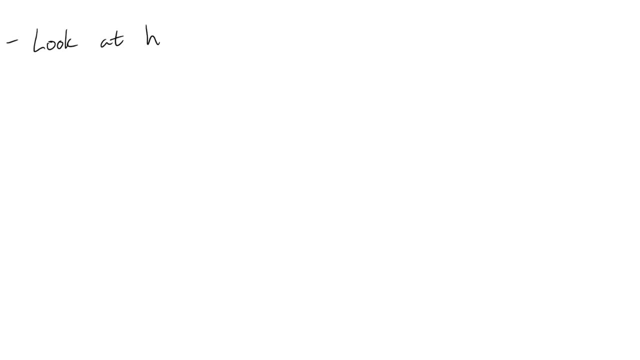 We can act on such a single particle state with the transformations of the Poincaré group, and the result will vary depending on the properties of the state. One such property is the spin of the particle. We can, of course, flip this logic around and instead: 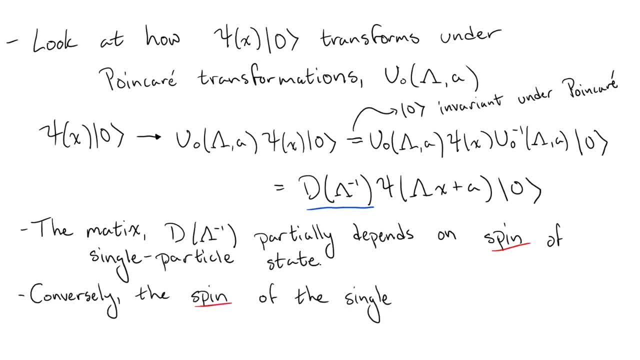 say that the spin of a particle is determined by how such a single particle state is affected by Poincaré transformations. This shouldn't really surprise us, because rotations live in the Poincaré group, The Poincaré group and, as we've already said, angular momentum. 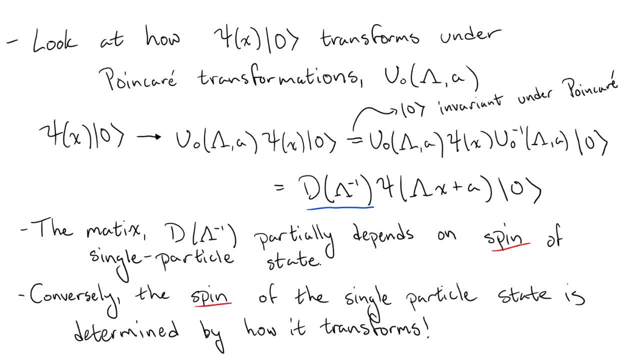 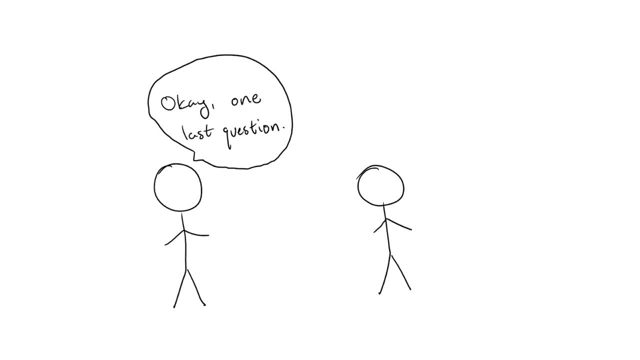 and therefore spin is deeply connected to rotations. Okay, so we've discussed what spin is and what determines a particle's spin, but there's still one more question about spin that's frequently asked: Why is it that fermions- particles whose wave functions are anti-symmetric, under exchange? 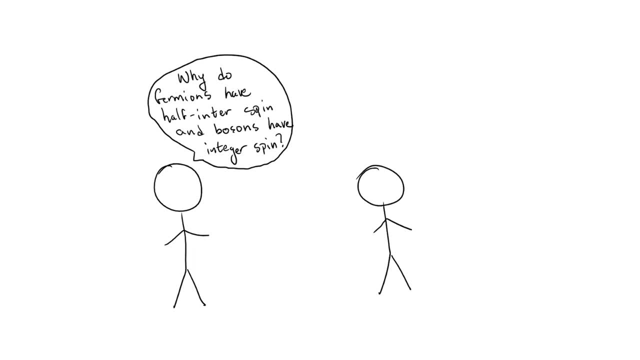 are always half-integer spin particles, whereas bosons particles whose wave functions are symmetric under exchange or integer spin. What's the connection between these symmetry properties of the wave functions and spin Incredibly? this is entirely due to imposing causality in quantum field theories. Causality simply means that no information can ever. 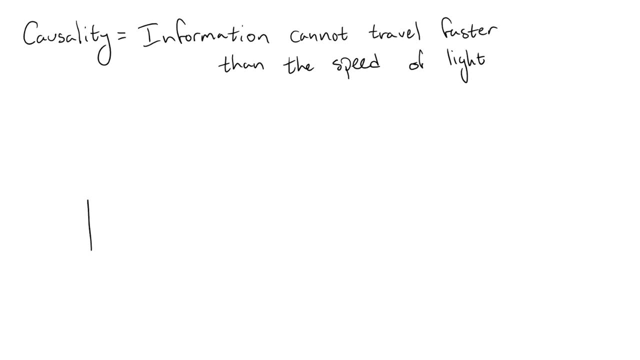 travel faster than the speed of light. If we have two spacetime points, x and y, separated in a way that a signal would have to travel faster than the speed of light to reach y from x, then the physics at point x can never affect the physics at point y, and vice versa. 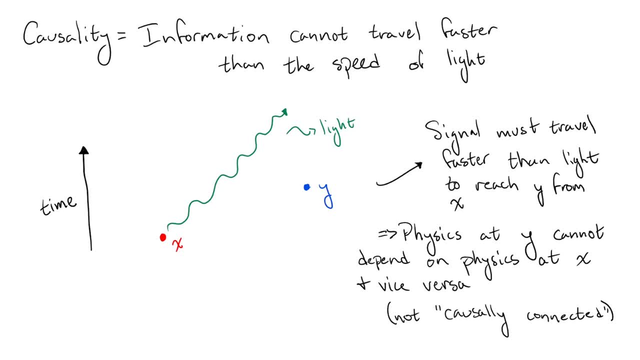 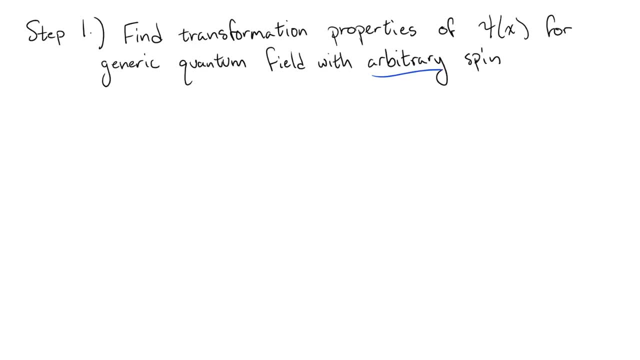 The mathematics of this requirement are quite complex, but the general idea is as follows: By studying single particle states, we can determine the spin properties of each of our fields. Then, by imposing causality, we can find certain requirements that our fields must satisfy in order to materialize. Causing causality is the process of determining the spin properties of each of our fields. Then, by imposing causality, we can find certain requirements that our fields must satisfy in order to materialize. And, finally, by identifying the spin properties of each of our fields.